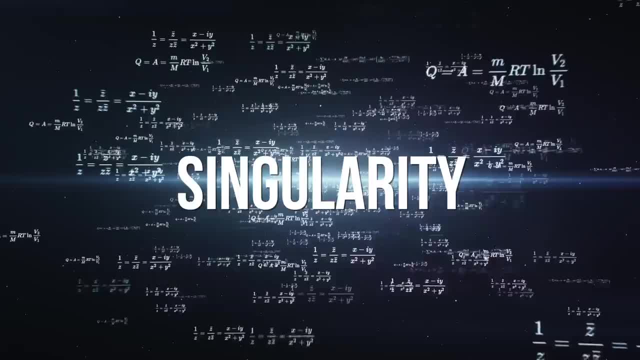 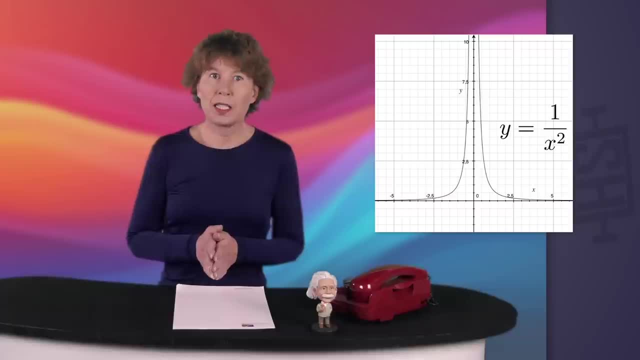 to what happened after, so we'd never know of it. To see what I mean, take a super simple example of a singularity: that in the function 1 over x squared when x goes to zero, It's not like there's no curve for x smaller than zero. it's just that there's no connection between the two. 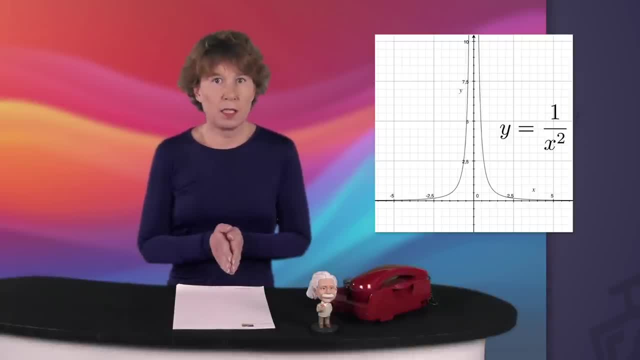 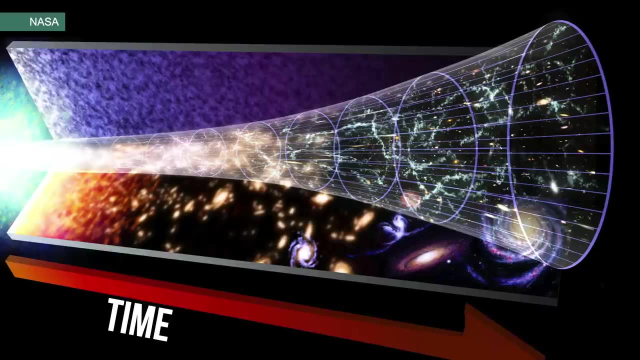 parts. The same could be the case for the big bang singularity. There was something before it, but it's not in any way connected to us, so we'd never know. That said, most physicists don't think that the singularity is even there to begin with. 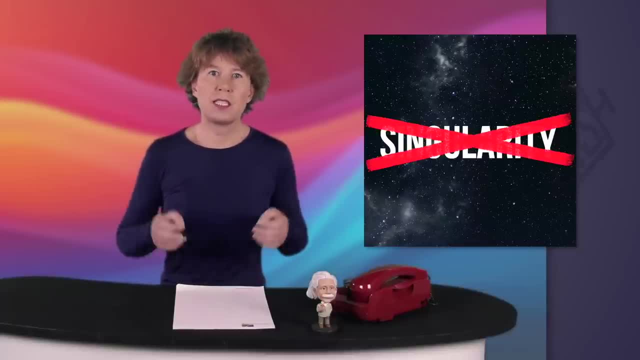 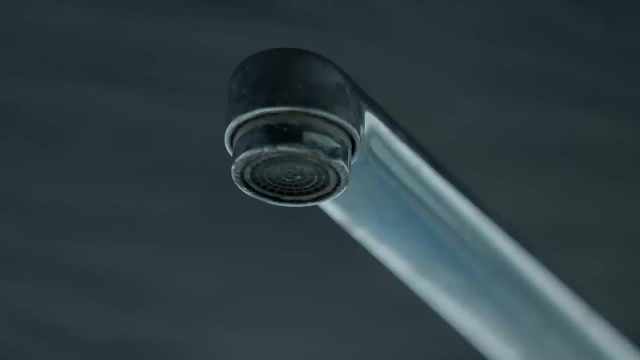 That's because in all other cases where we have a singularity in a physically measurable quantity, it just means that the theory breaks down and we need to use a better one. A good example is hydrodynamics. that describes how liquids behave. Surfaces of drops can have points with infinite curvature. 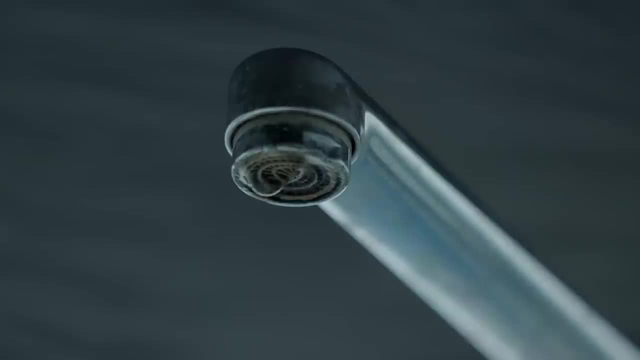 like when a drop of water pinches off a tap. That pinch-off point is the singularity. But of course, if you look at the drop on the scale of a single atom, there's nothing singular about it. It's just that if we approximate all those atoms with a smooth 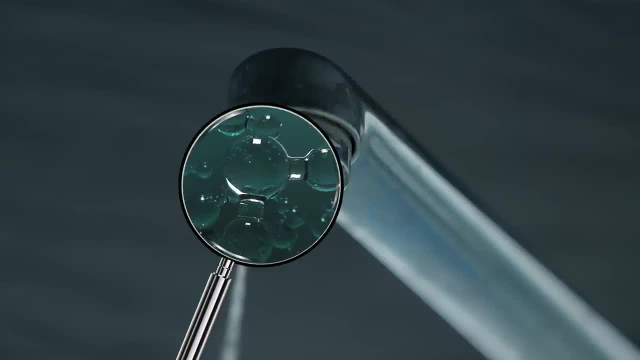 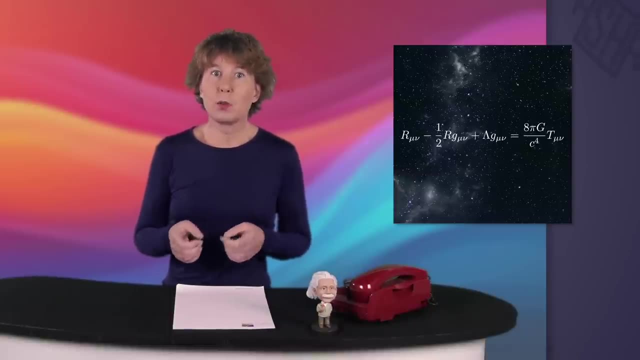 fluid that those singularities appear. they're a consequence of this improvisation. That's why physicists think the Big Bang Singularity just tells us that we need a better theory. We don't have that theory, so the smart thing to do would be to leave it at that. 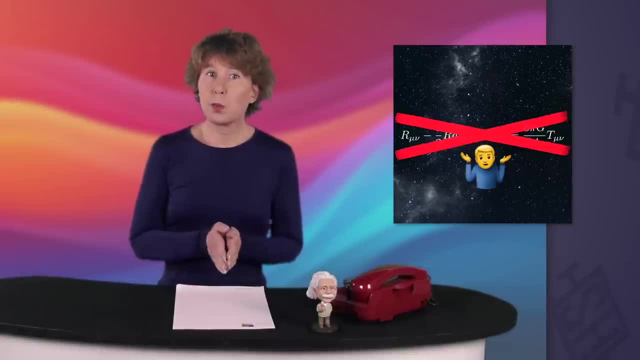 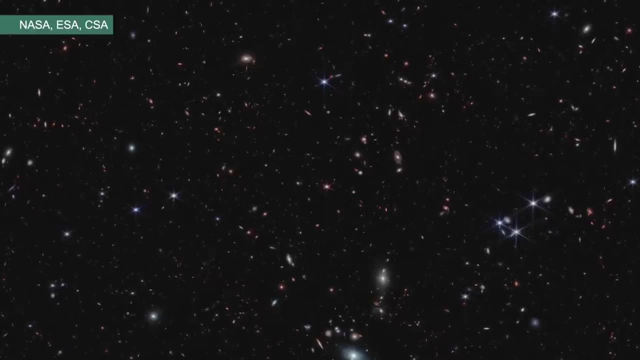 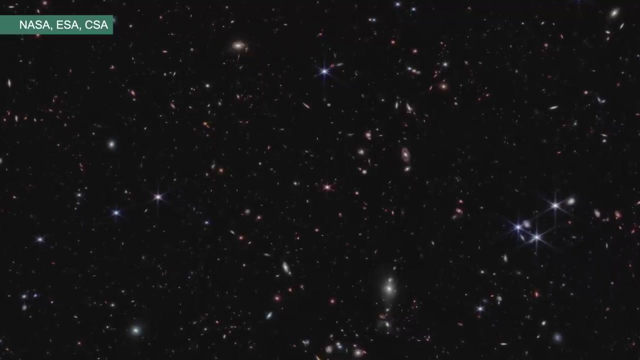 But that's no fun. so physicists have come up with a lot of speculations for what might have happened instead of a Big Bang singularity, And there's very little data in the way of their speculations. The young galaxies that the Webb telescope sees were probably created a few hundred million years. 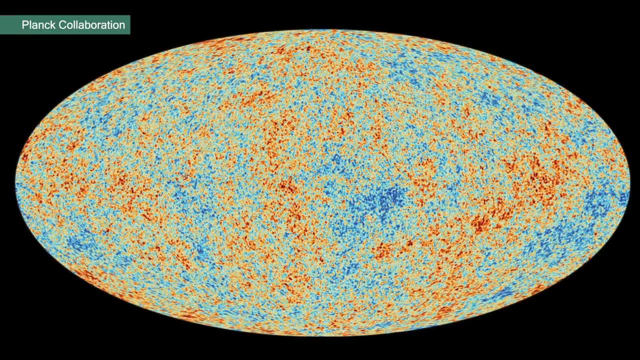 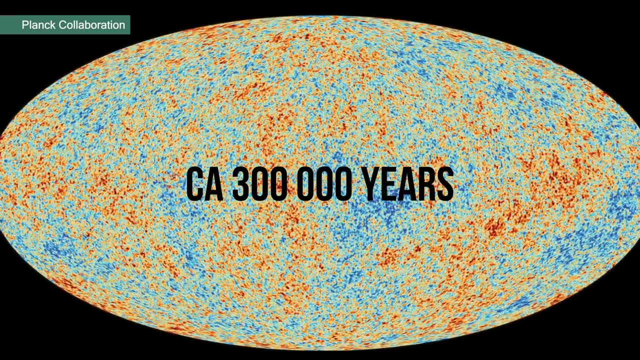 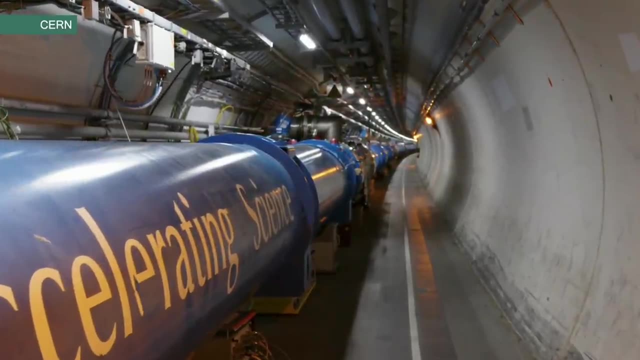 after the Big Bang. The cosmic microwave background was created approximately 300,000 years after the Big Bang and we have no observations from earlier on. Physicists have used particle colliders to study what highly compressed matter does, and we can use this data to extrapolate back to somewhat before the creation of the cosmic. 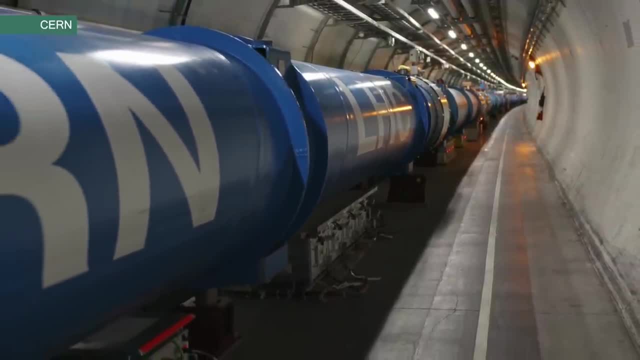 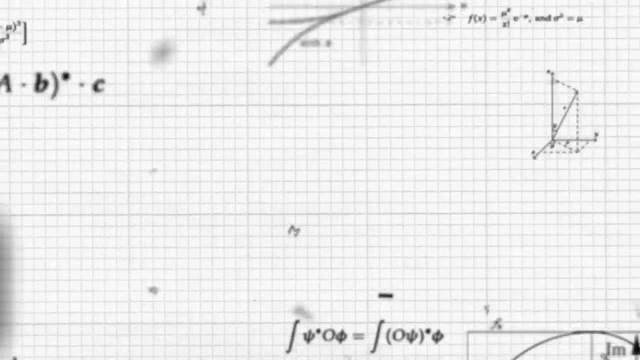 microwave background to around the time when the Higgs field condensed, But this still doesn't get us anywhere near the Big Bang. This is why in theoretical physics you find many alternatives to the Big Bang, And this is why we have no observations from earlier on. 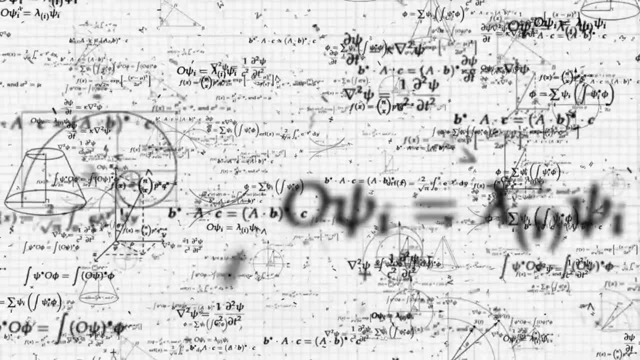 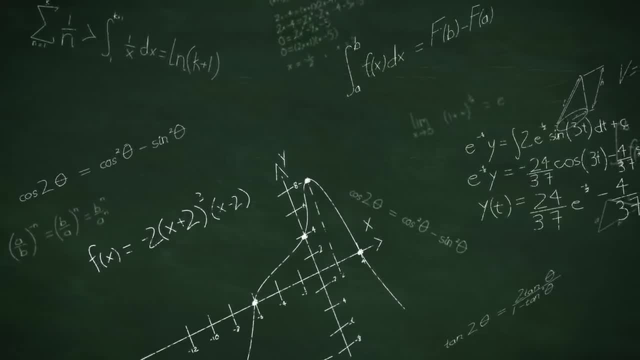 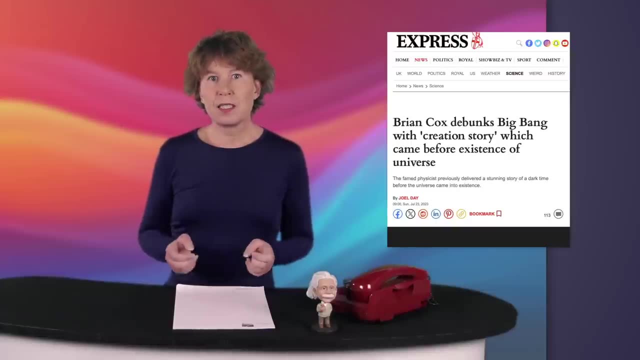 Alternative ideas for the beginning of the universe, depending on how you change the equations, because there's no data to tell those ideas apart. And this brings me back to Brian Cox's supposed debunking of the Big Bang. In this clip from the BBC, he's clearly talking about the 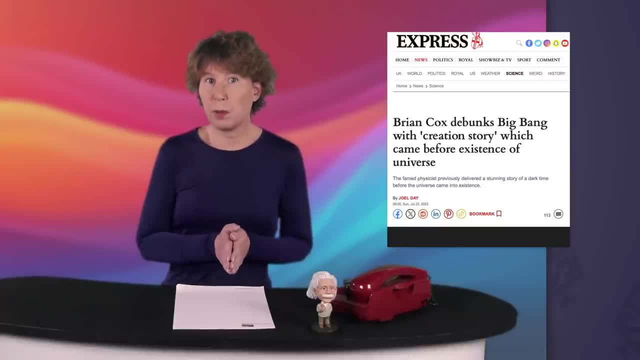 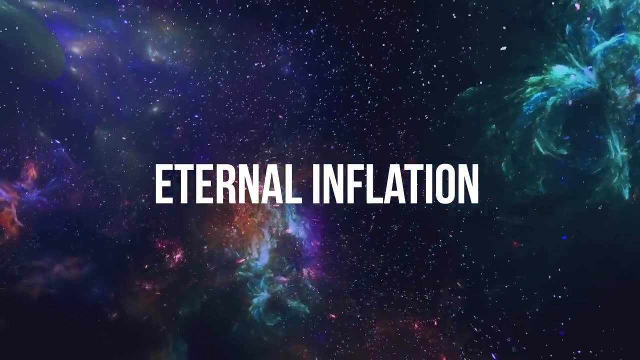 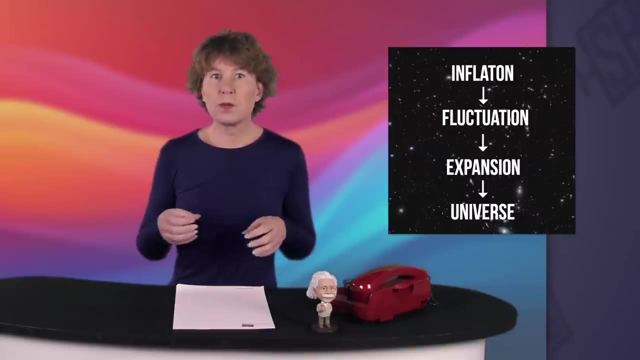 currently most popular theory for what happened before the Big Bang. It's called eternal inflation. In eternal inflation, the creation of our universe is not singular, so, strictly speaking, there isn't any bang. According to this theory, our universe is created by a quantum fluctuation in a field called the inflaton. The inflaton creates this. 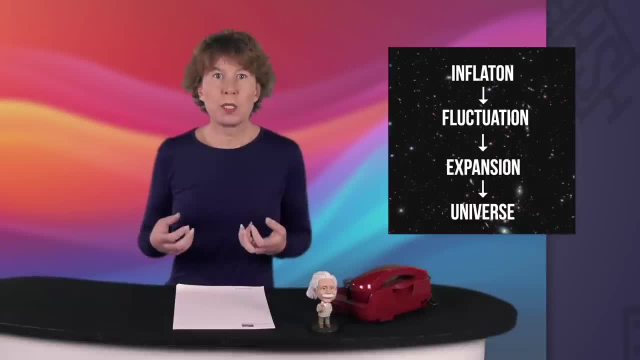 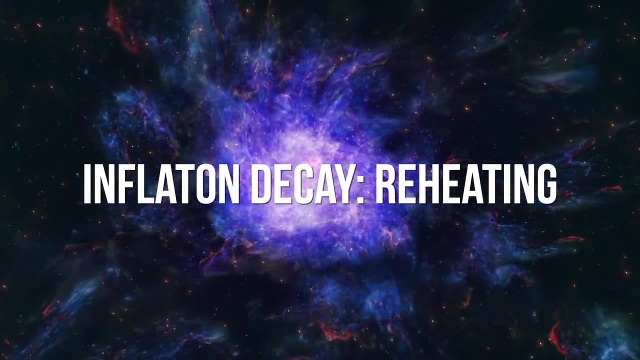 fluctuation and that creates a bubble which then rapidly inflates, hence the name. At some point the inflation stops and all the energy from the inflaton field is converted into matter. All the matter around us is created only at that point, when the inflaton field dumps its energy. 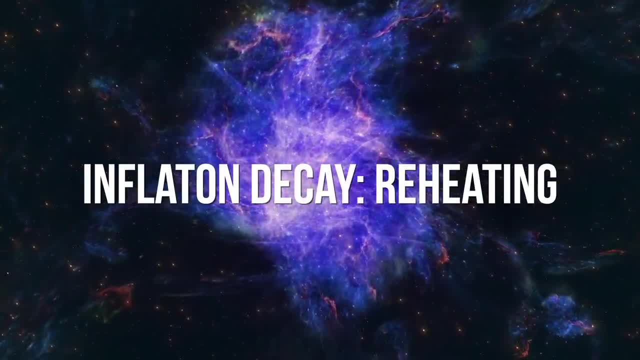 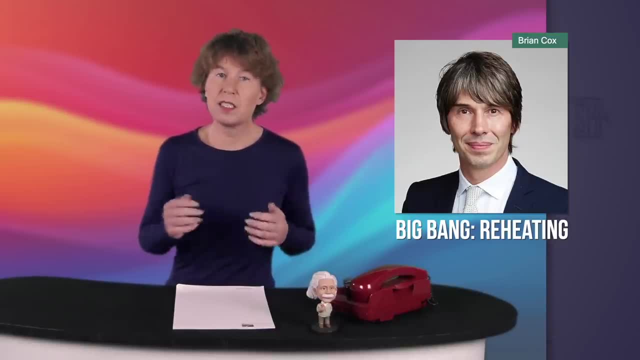 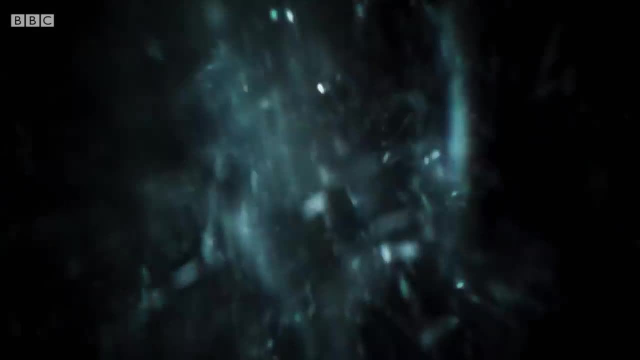 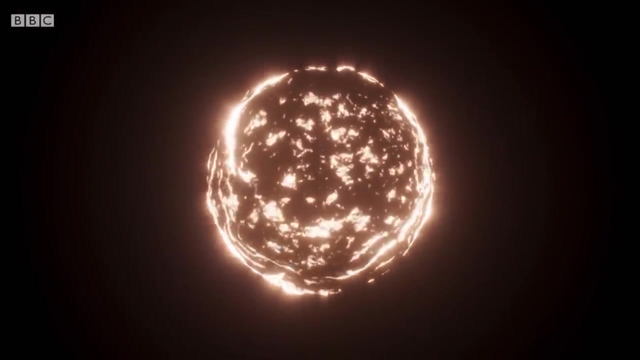 In the literature, this event is usually referred to as reheating. What happened with Brian Cox's explanation is that he made it sound as if the reheating is the Big Bang. I mean, listen to it yourself. So basically he just used the word Big Bang for something completely different. 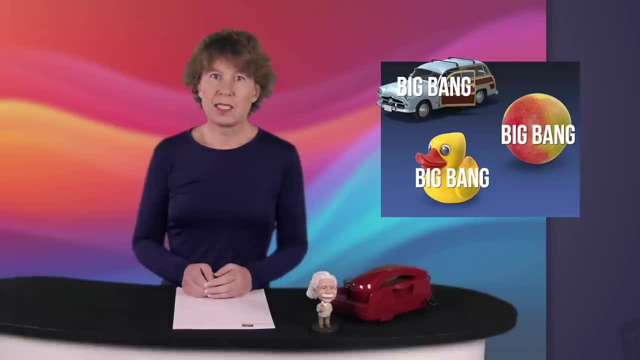 It's somewhat of a disease among science communicators that I've complained about before, because it causes a lot of confusion, but let me not go there again. Maybe more importantly, even leaving aside that we don't know whether eternal inflation is even correct. 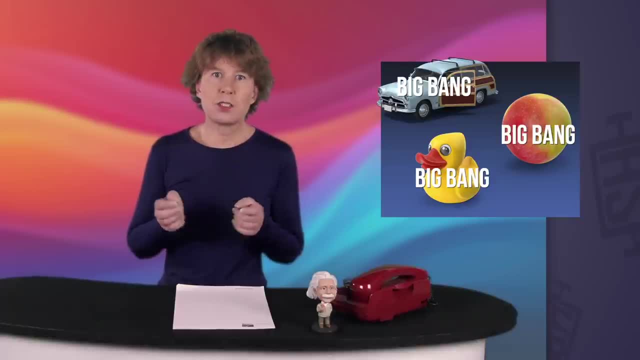 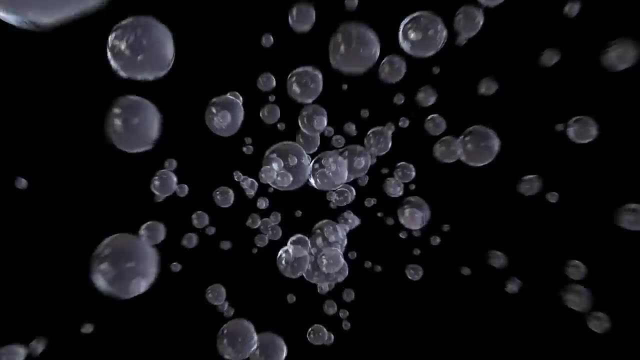 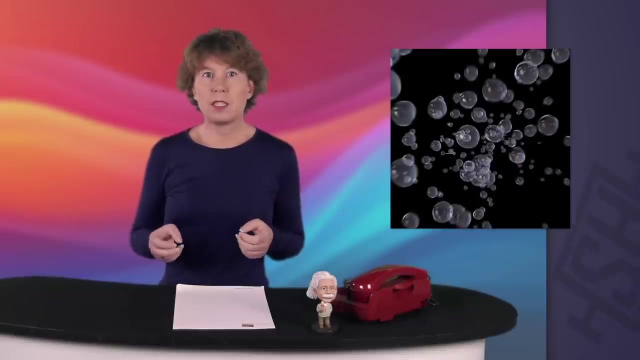 it doesn't remove the Big Bang per se, It just removes the Big Bang in our universe. You see, in eternal inflation there are infinitely many of those quantum fluctuations and each gives rise to a new universe, This entire multiverse of eternal inflation. however, 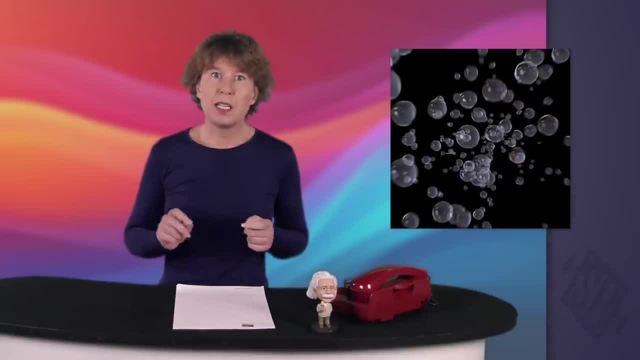 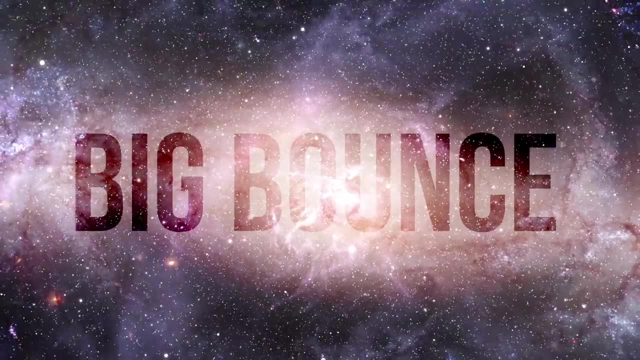 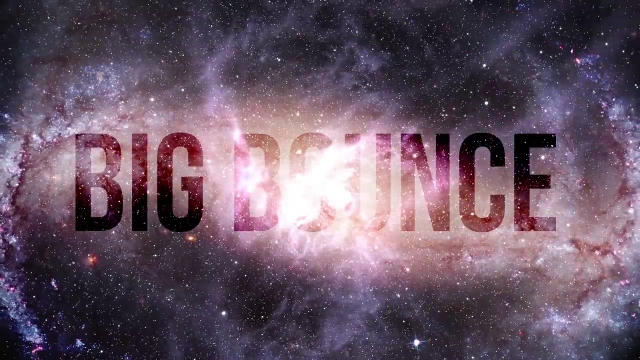 must also have had a beginning at finite time, and then you can ask: well, what happened before that? So eternal inflation just moves the problem elsewhere. And of course there are other ideas for the beginning of our universe besides eternal inflation. For example, there's the idea of a big 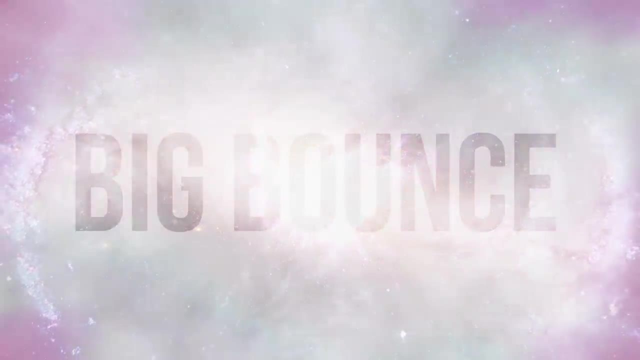 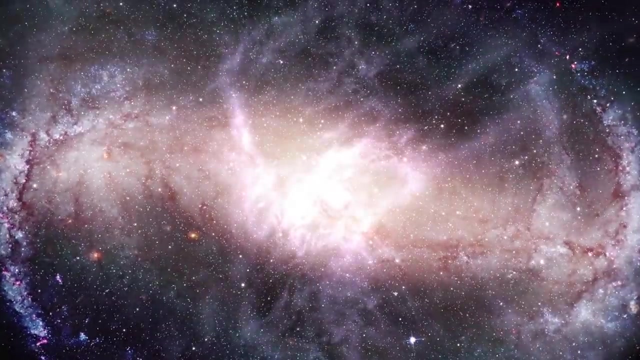 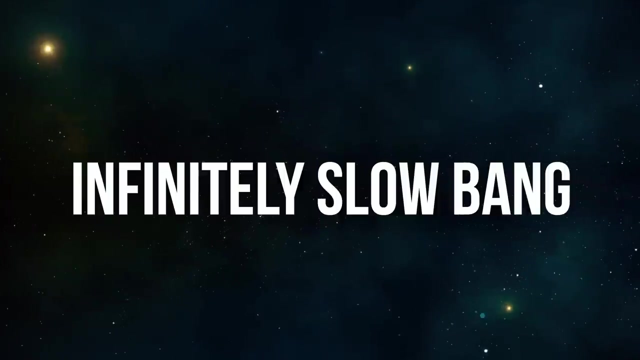 bounce in which there was an earlier phase of the universe which contracted. Matter became very dense, but not infinitely so, and now it's expanding again. If those bounces repeat, it's called a cyclic universe. You can also just push the Big Bang all the way back to minus infinity and say: 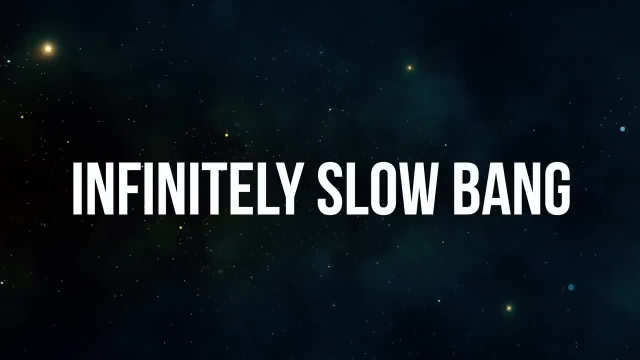 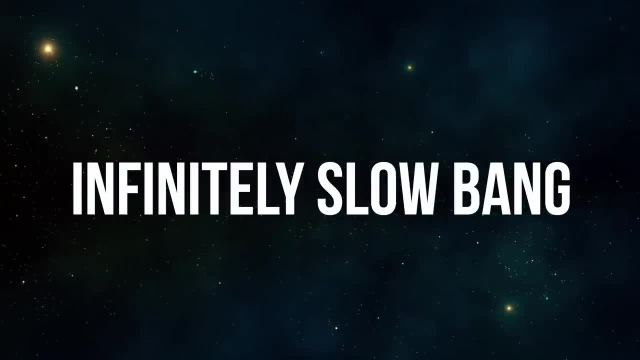 that for half of infinity very little happened and then the universe suddenly started expanding. It's not a very popular idea, probably because the entire point is that it's infinitely lame. Or there's the Hartle-Hawking no-boundary proposal that says before the Big Bang. there was no space-time, there was just a four-dimensional space, and then one direction of that space turned to time. These ideas are all more or less compatible with observations, because you can always make sure that the deviations from Einstein's equations are unmeasurably small. This doesn't mean these ideas are wrong. it's that we can't tell whether they're. 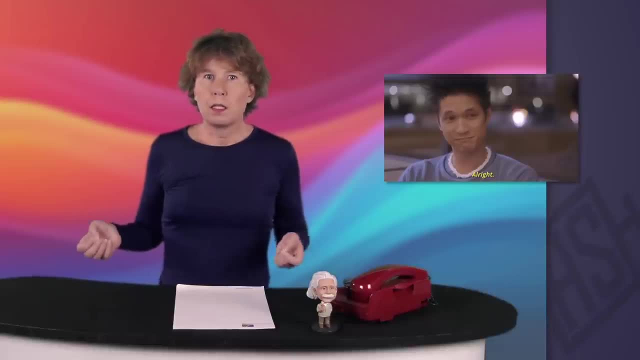 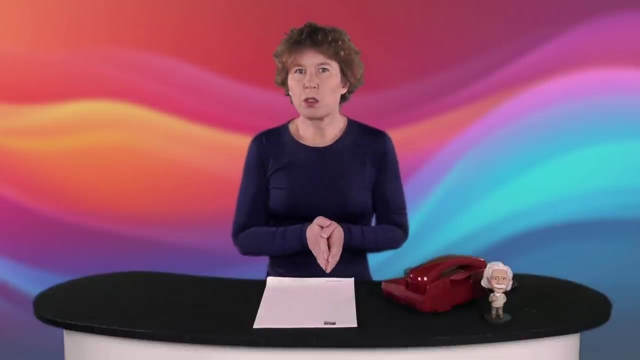 right or wrong. So what happened before the Big Bang? Physicists have a lot of speculations, but the short answer is that we don't know, And since there's so little information left over from whatever happened, we might never know. So it's not like Brian Cox said something wrong. 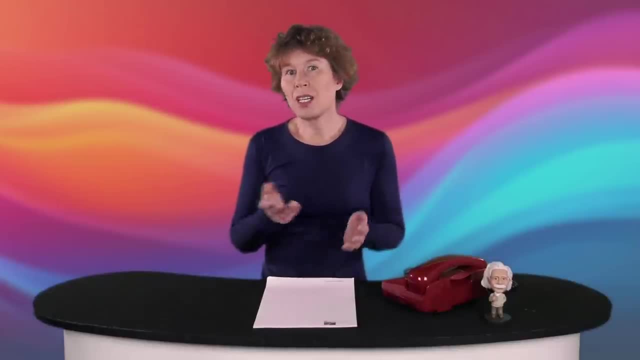 it's just that communication is difficult, Which is why I always try to learn a few words in the local language when I'm traveling. As I've mentioned before, we're planning to go to Paris and I've been learning some French with Babbel, who've been sponsoring this video. I've made some 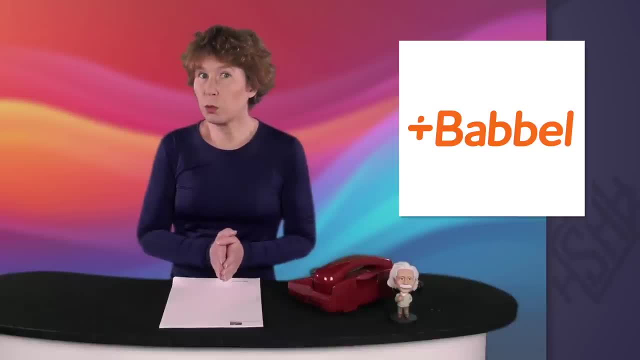 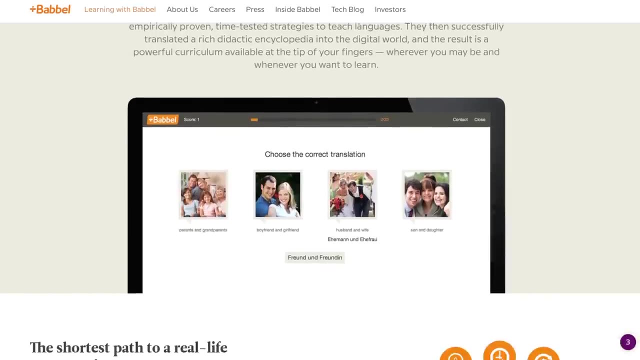 little French mistakes, Excusez-moi. quel âge a l'univers? But let me tell you something about Babbel first. It's one of the most widely used language learning apps in the world, and that's for a good reason. It's super easy to use, works on your phone or your browser. 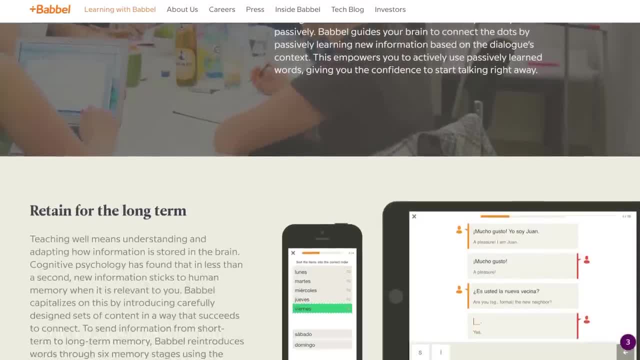 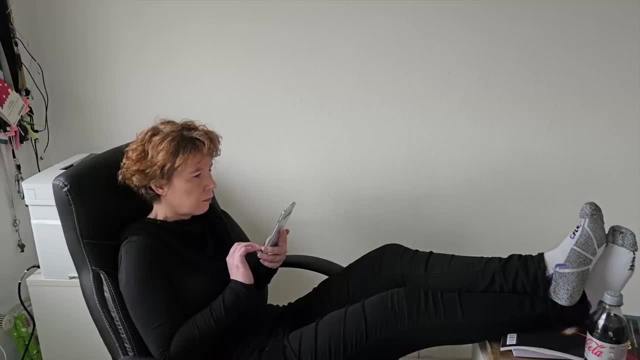 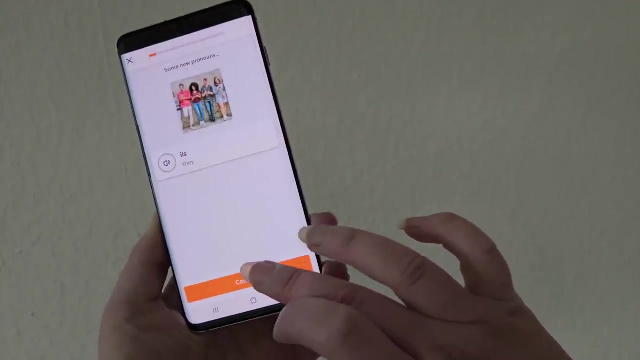 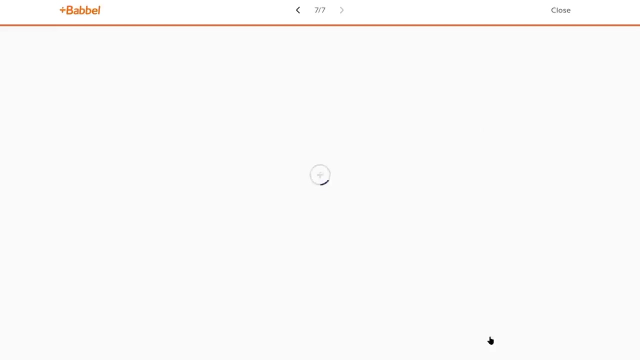 and gets you to your goal quickly. Their lessons are designed by language teachers and you can complete them step by step whenever you find the time. The best thing about Babbel is that it teaches real-world conversation, For example, how to sort out travel problems or talk about business matters- stuff you actually need. 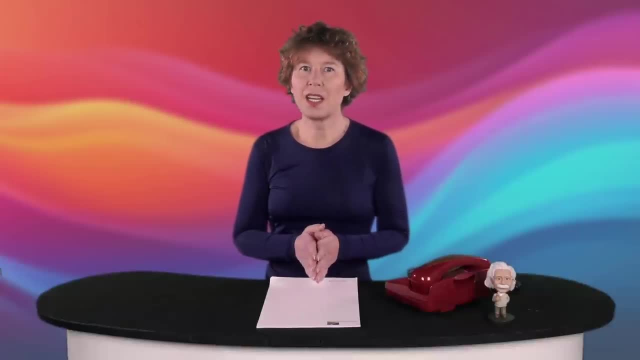 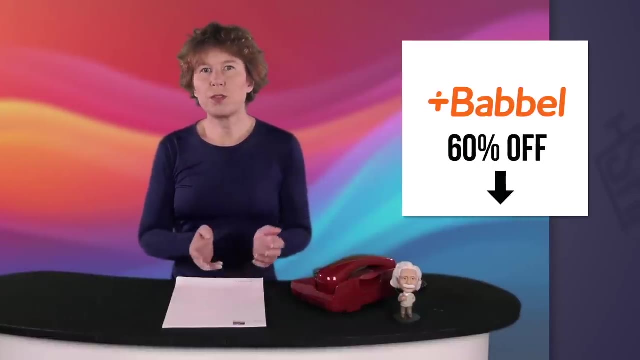 And I have an amazing special offer for you today. If you use our link in the info below, you'll get 60% off your subscription And don't worry if you don't like it, you have a 20-day money-back guarantee. So go and check this out.